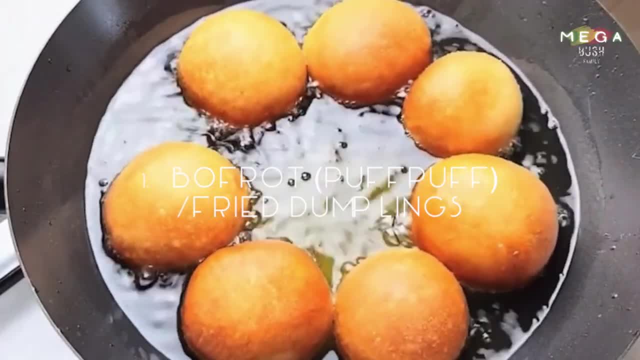 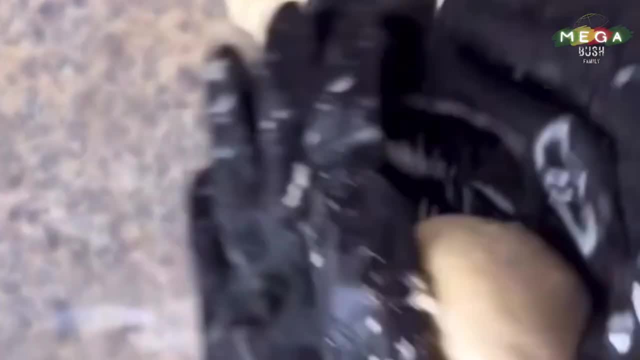 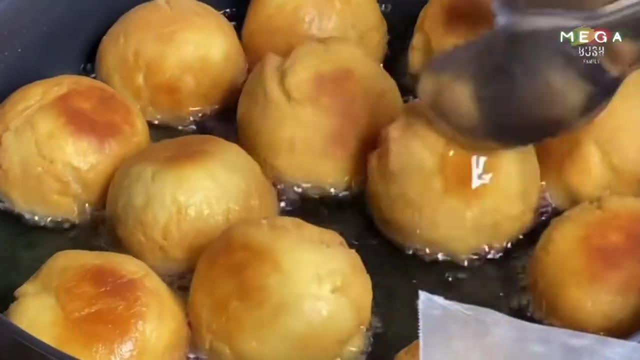 list is buffroot. i hope i pronounced that correctly. it's also called puff puff. now every Jamaican watching this is saying: no man, then this on a dumpling. yes, in Jamaica we call puff puff fried dumplings and we usually have it with um acan, salt fish or any other delicious side. 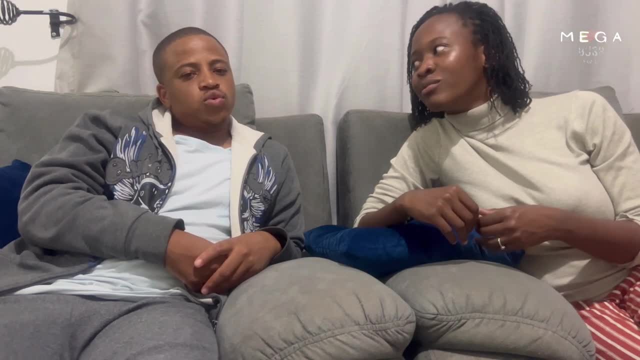 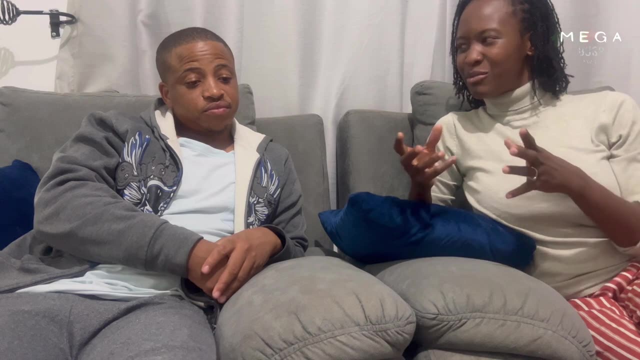 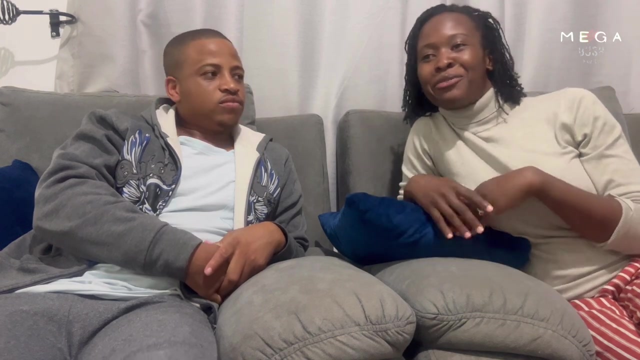 the stimulus is something we call fat cooked or margarita. you don't eat like a jealous dude. okay, yes. so in Ghana they seem to eat it alone. yeah Well, Jamaicans will like to spice things up, so we eat it with relish, which is usually 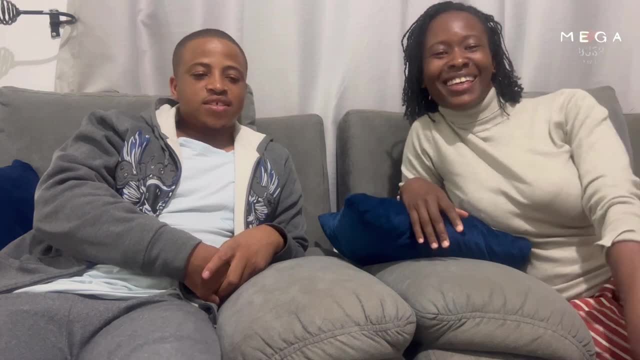 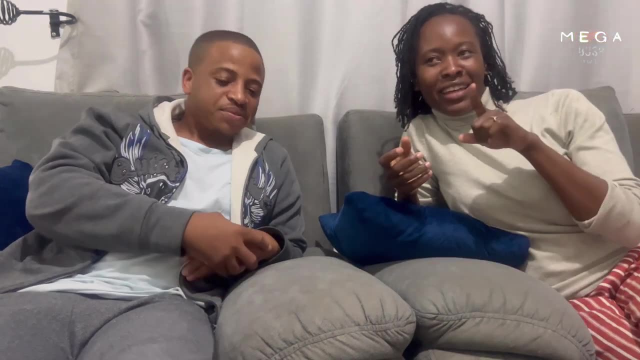 ackee and salt fish or really anything else. Oh, it's extra Jamaican, extra, extra, extra. All the Jamaicans. please shout out in the comments below: Alright, so yeah, that's Puff, Puff. and the second thing: you don't like this. 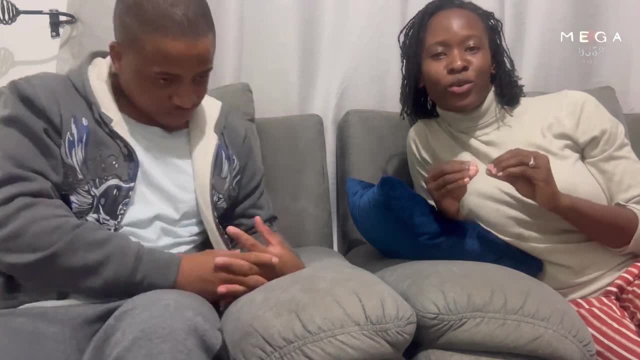 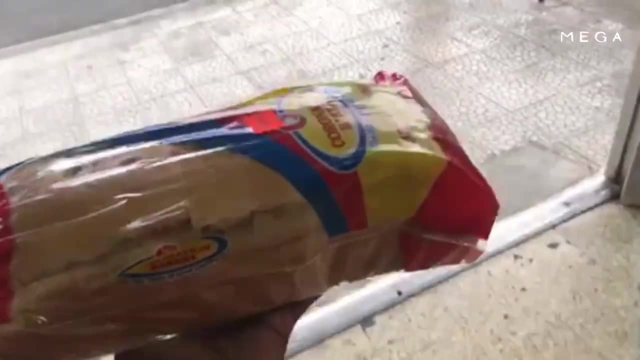 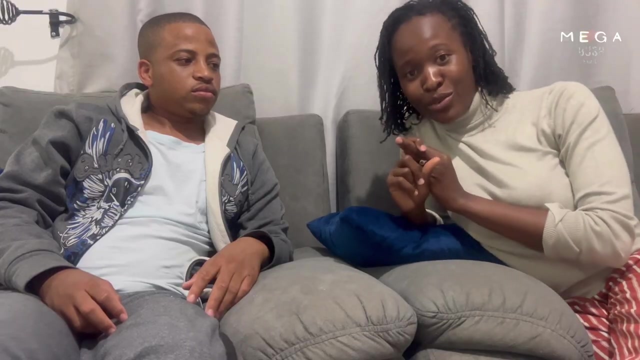 He doesn't like this. In Jamaica we call it hard dough bread, So hard dough bread is a staple in every Jamaican household. What makes it unique is its dense texture. Imagine my content when I found a similar bread in Ghana. I brought home three of those loaves and I thoroughly enjoyed them. 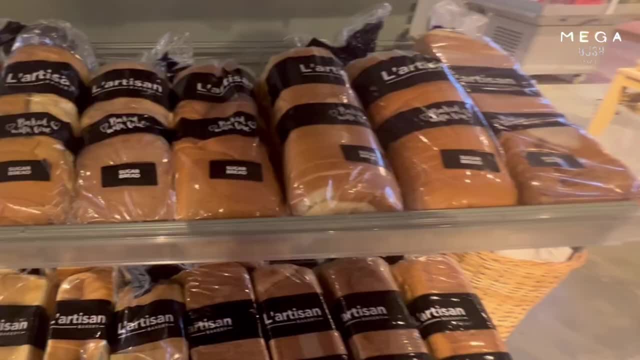 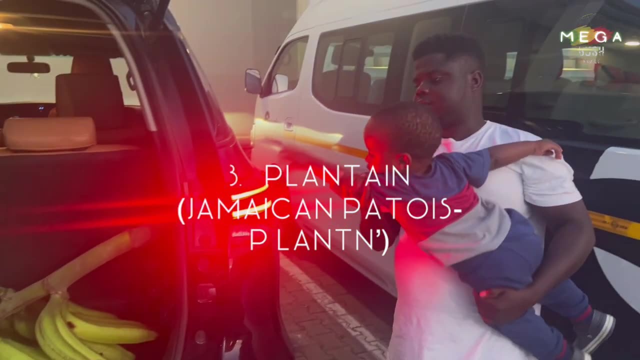 We've been to a number of different countries and this is the first country other than Jamaica that I was able to find hard dough bread. Similarity number three and my most treasured takeaway from Ghana: plantains. Between Jamaica and Ghana there are a lot of different kinds of plantains. 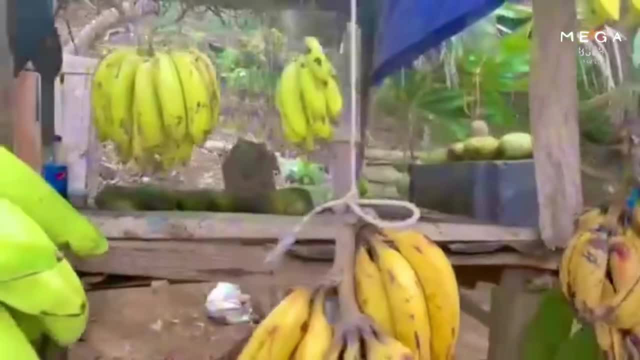 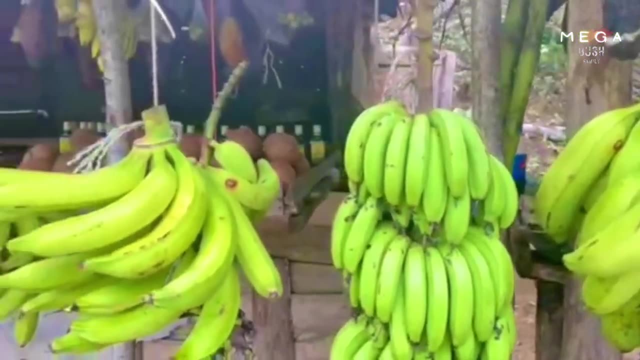 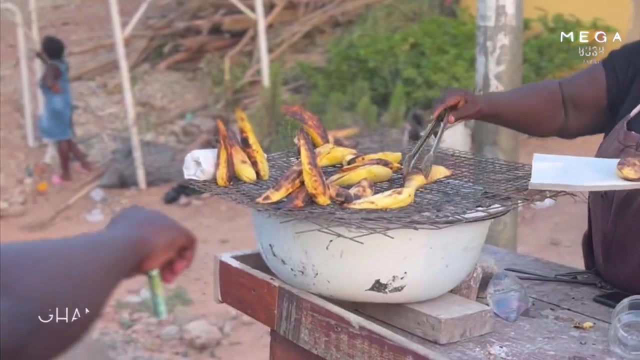 For Jamaicans and Ghanians. I'm not sure who loves plantains more, but driving through Jamaica, you will find plantains like these hanging by the roadside being sold almost everywhere. It's a food we love, Bless. In Ghana, you will find plantains by the roadside as well, but most times they're roasted or 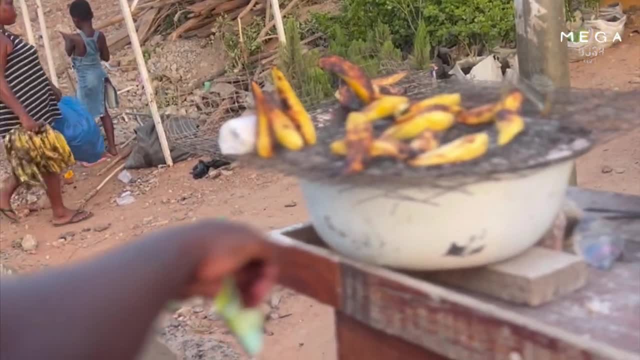 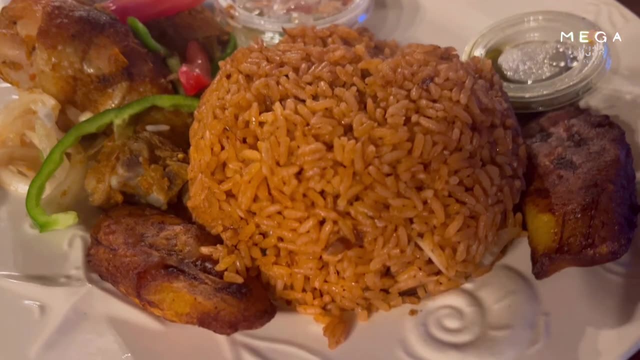 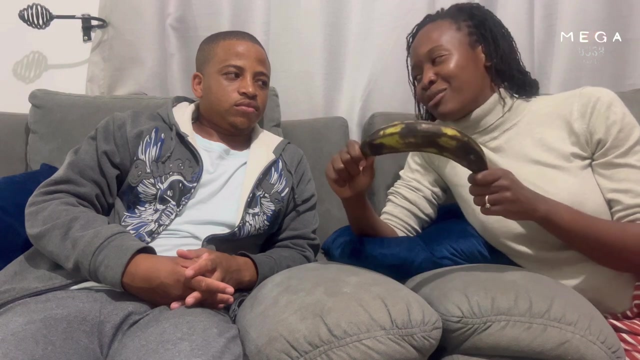 in the form of fried chips. I'm from here, What are you from? Because I want, Just like Jamaicans, Ghanians like to have fried plantains as a side and it's just as tasty. This is one of the leftovers that I brought to Zil from Ghana. 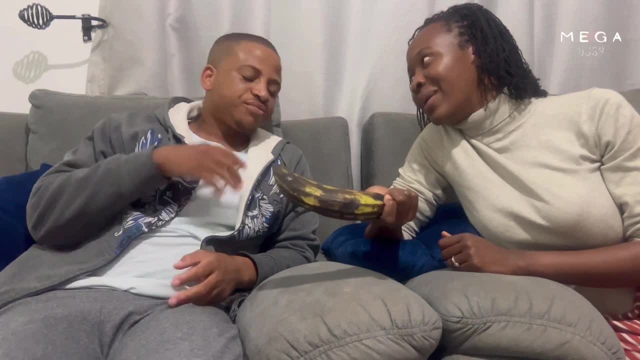 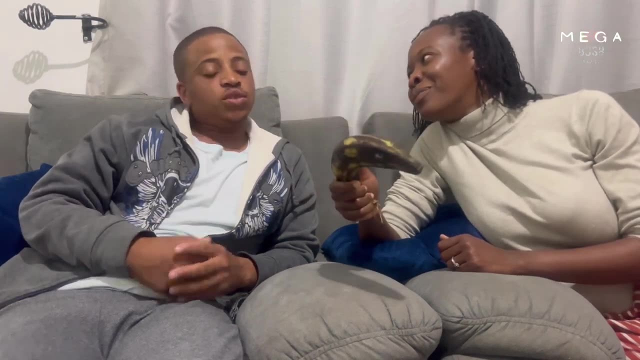 Initially you didn't like plantains, right? Nope, But you like them now, right? I told her this, but no, I didn't. Unfortunately, plantains aren't grown in Zimbabwe, so Tony may never get the chance to come to love them. 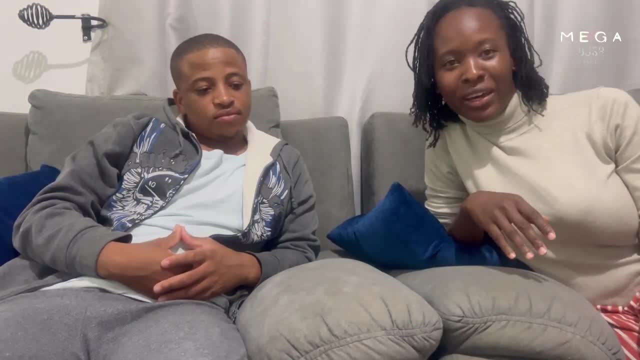 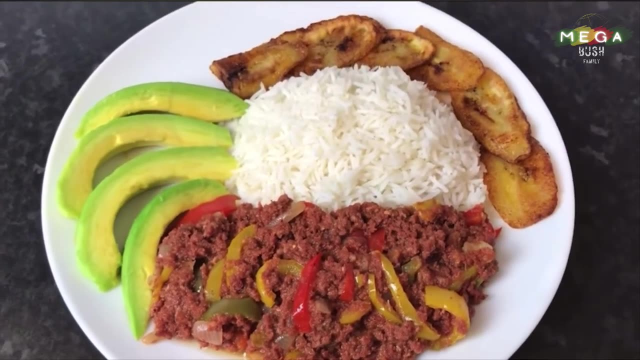 So the fourth thing is something we call bully beef. in Jamaica This is a meal that's cooked in olive oil Almost every Jamaican household, And I'm sure a lot of Jamaicans thought we were the only ones who eat corned beef, and 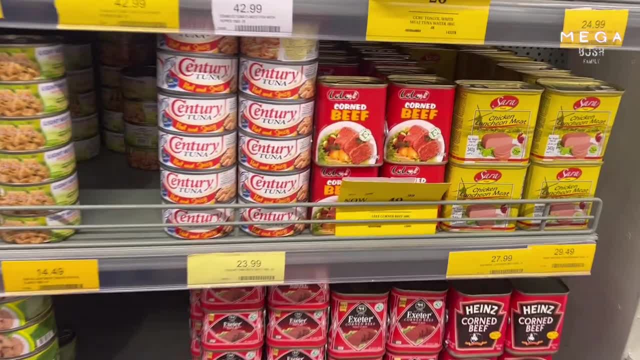 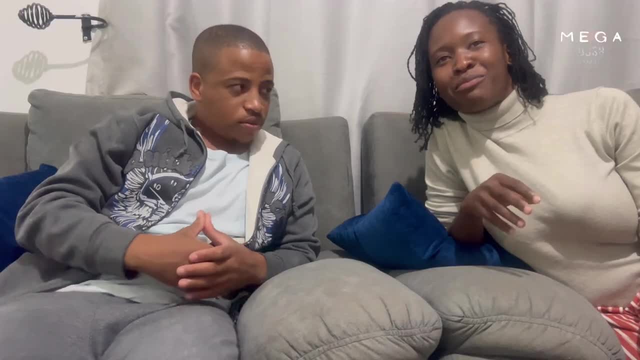 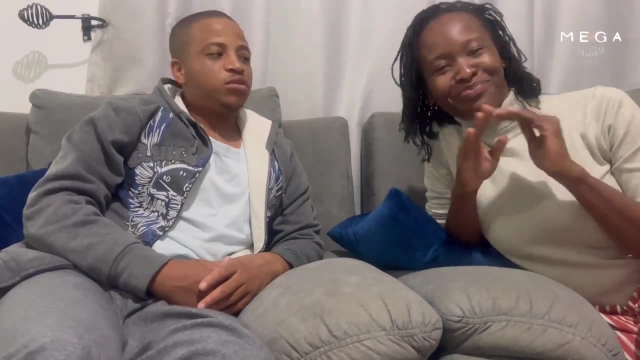 rice, Nope, So do Ghanaians in exactly the same way. Yeah, corned beef in a tin with that key like we turn and open it. If you ever lost that key you'd be in trouble. You need to look for a knife, or 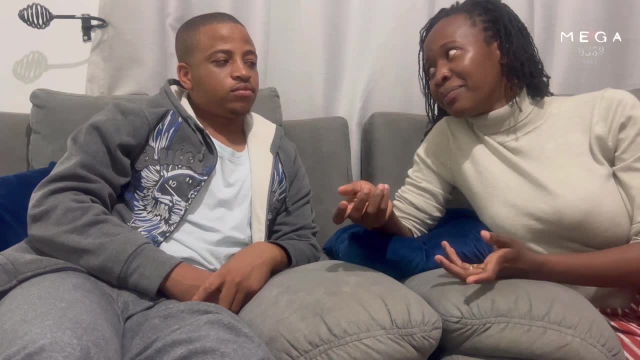 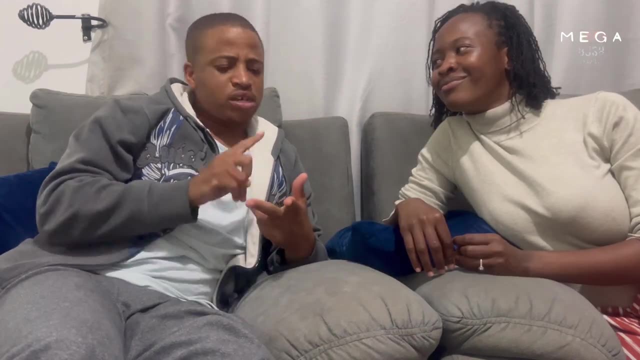 Trouble sometimes. Anyway, We tried it here in Zil Yes, And It wasn't the same. When it comes to, like you know, meat products, especially beef and chicken, I think Zimbabwean quality is the best And 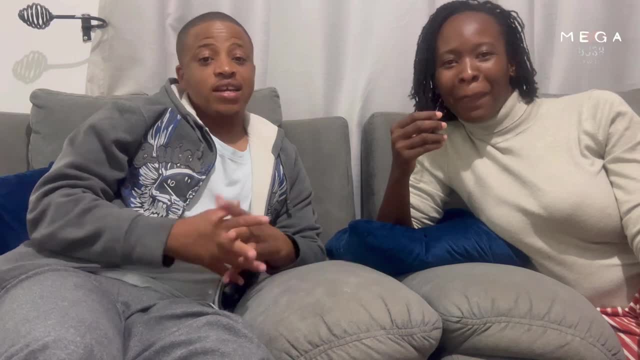 This is a discourse for another video: Zimbabwean beef, especially Zimbabwean beef. You have to try it. Yeah, it's okay, I give it to Zimbabwe. I think I agree Their steak top tier. I think Zimbabwe is the best. 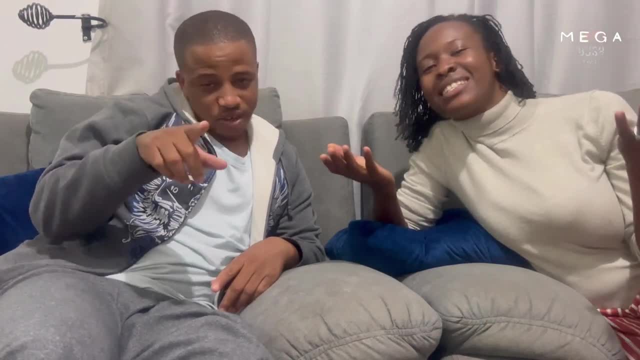 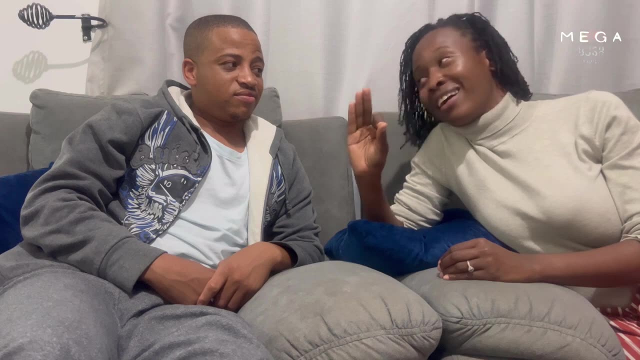 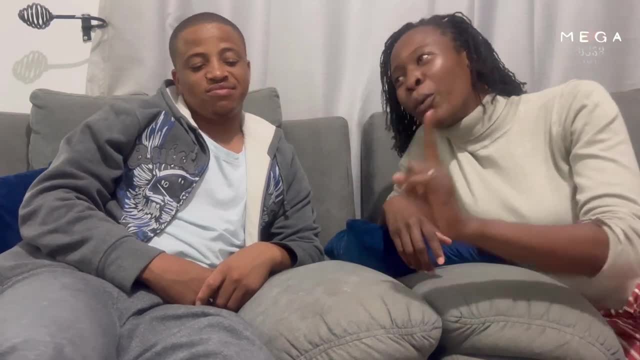 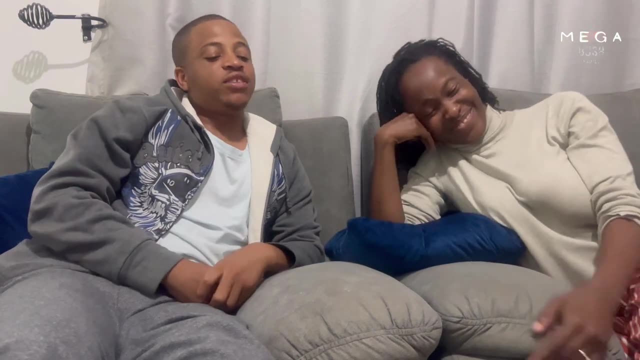 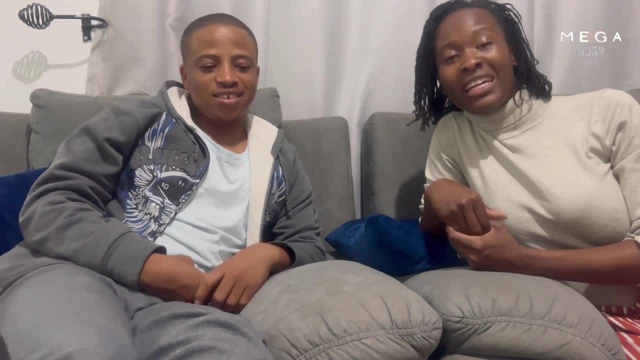 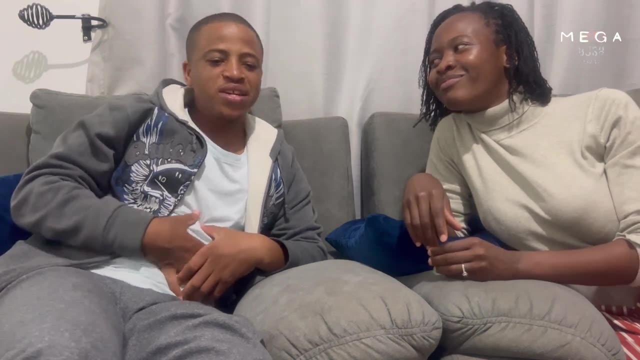 You love shito? right, Yeah, I love shito. Good food, Yeah. he kept asking before he did every restaurant: can I have some shito? Yeah, but it made my tummy funny. I always used to ask him: when is this going to stop? He's like: no, your tummy will get used to the shito, So just keep going. But I love shito Much like our Ghanaian family. Jamaicans love to cook with a lot of spices. We often marinate in a number of different seasonings to bring out the flavor in our food. 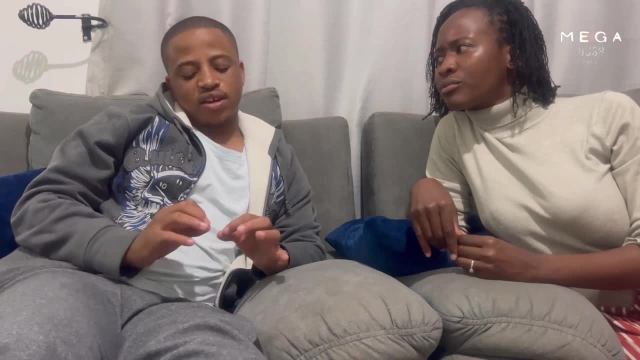 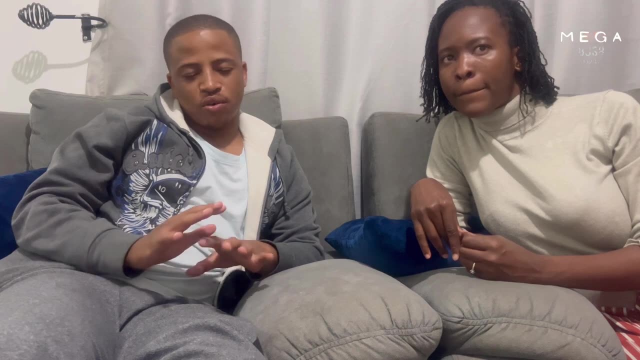 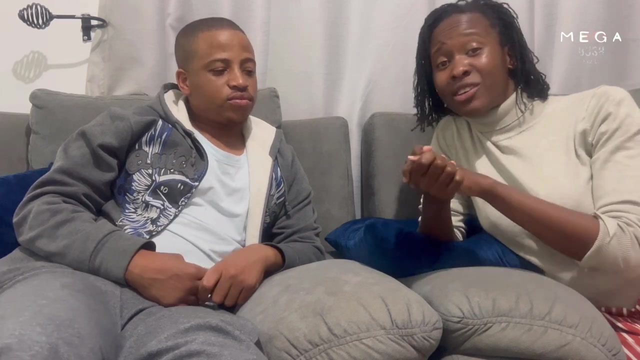 We're in Zimbabwe, I think We use a narrow variety of spices- Spices we're used to and we stick to that- And we tend to like our food more to be natural, almost soft cooking If you taste their food like a rosé. 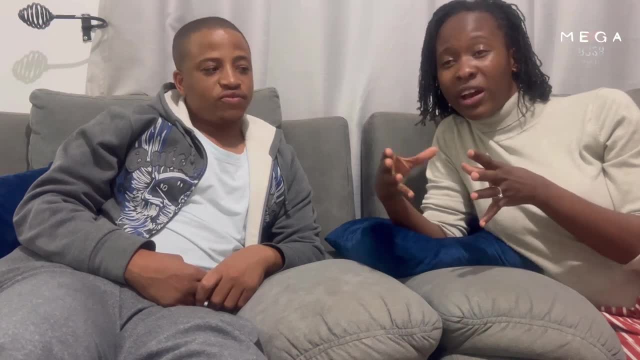 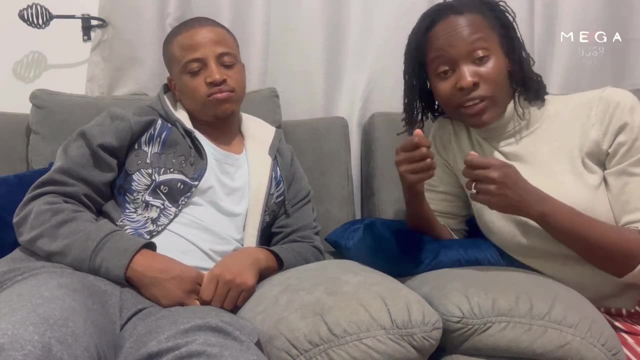 a groundrunner stew, that food that's cooked over the wood fire. they don't add any seasoning to it. It's just like onions and tomatoes, but it's so flavorful. So Zimbabweans can really cook without you know adding too many spices. 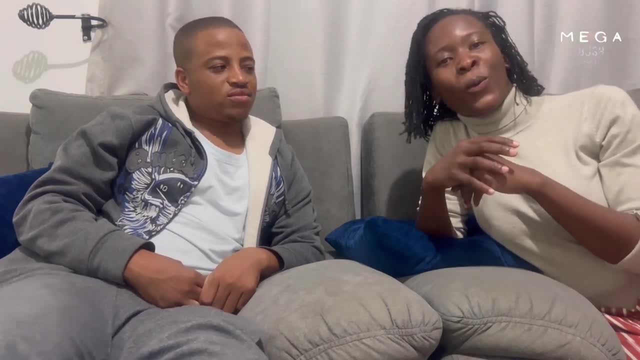 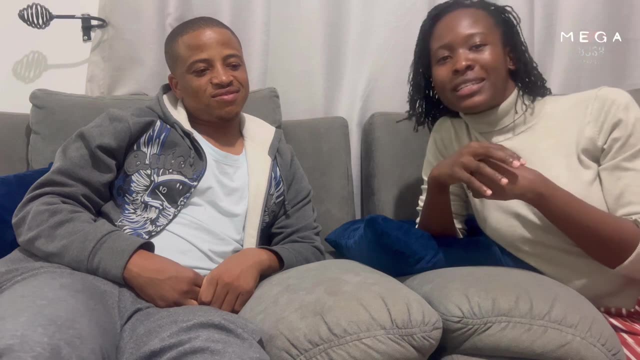 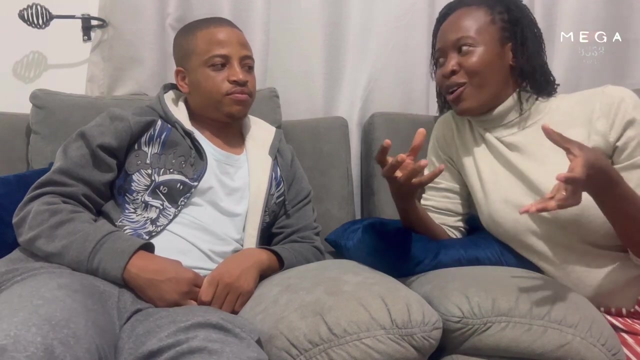 But us Jamaicans and Ghanaians, we love our spices, Ghanaians love them. pepe, We love our all-purpose and our onion, our thyme and everything chopped up, And So I thoroughly enjoyed the flavor of all the foods. 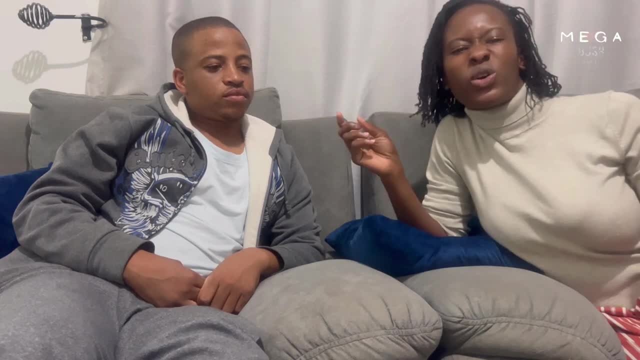 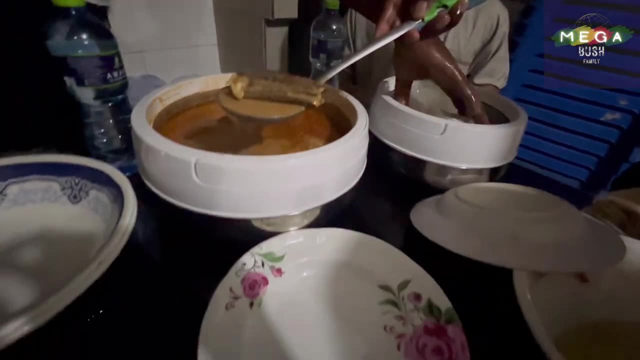 And I think that's a similarity between Ghanaians and Jamaicans: We cook with a lot of spices, While in Ghana we ate from a lot of different places, But the highlight was Auntie Maggie's fufu in groundnut stew. 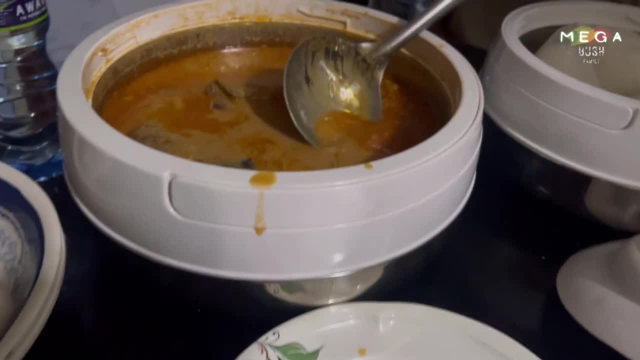 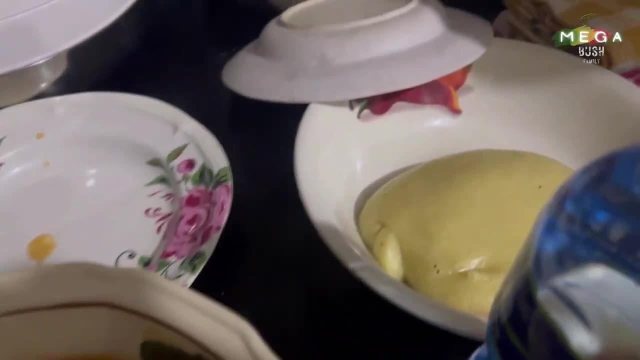 Groundnuts, Groundnuts, Groundnuts, Groundnuts, Groundnuts. I like that. Yeah, that one just tastes like fufu. I'll put it on this one. Hm, I'll put it on this one. What's that? 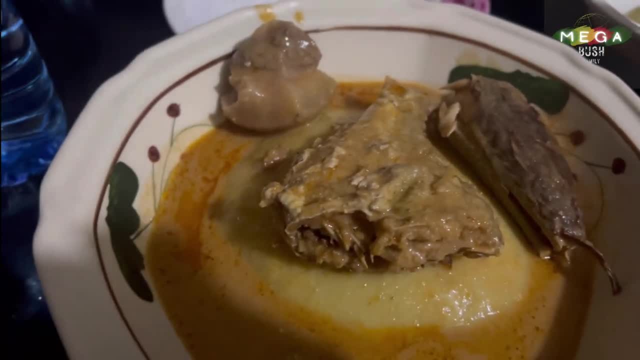 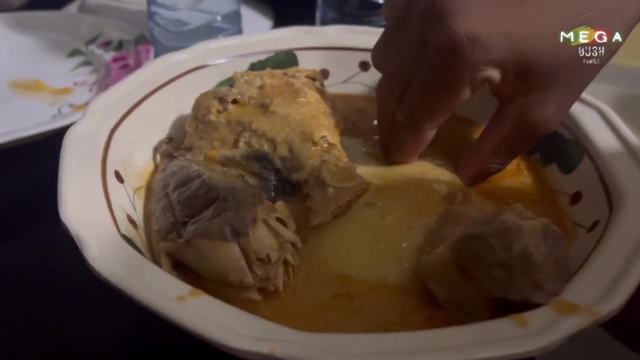 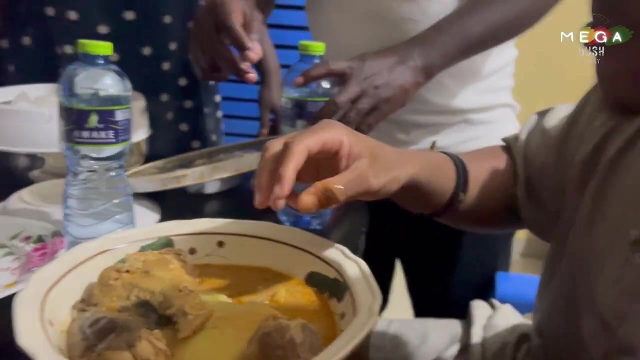 Something from the cup. It's snail, It's snail. Side note, We did struggle with the concept of not chewing. fufu Like submarine, Don't chew bro. No way It's on chewing. You gotta not chew it, man. 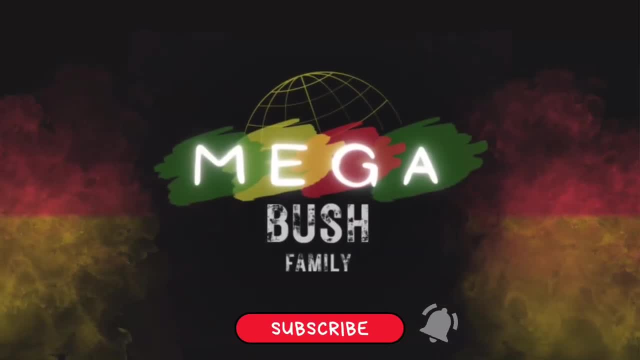 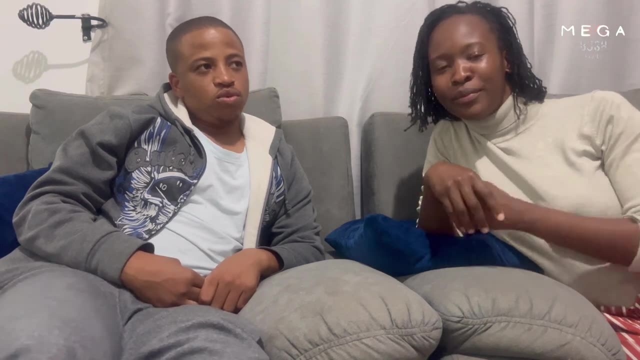 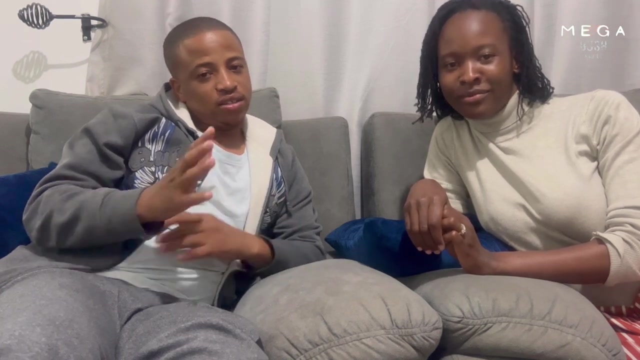 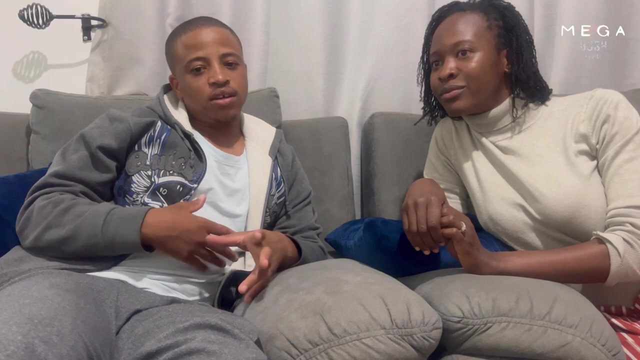 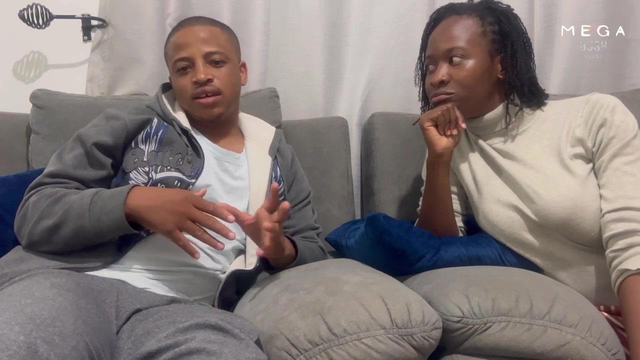 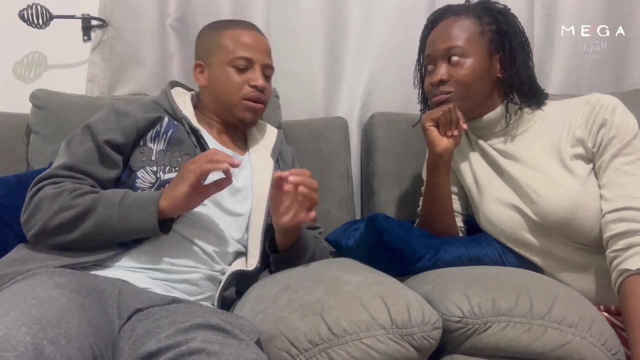 If this is your first time watching, please do like and subscribe What We in the southern part of Africa or East Africa, If you go to maybe study for- we've done, coming down and done the Tanzania, Kenya, Malawi, Zambia- probably Our dishes. they differ a bit but they're more or less the same.